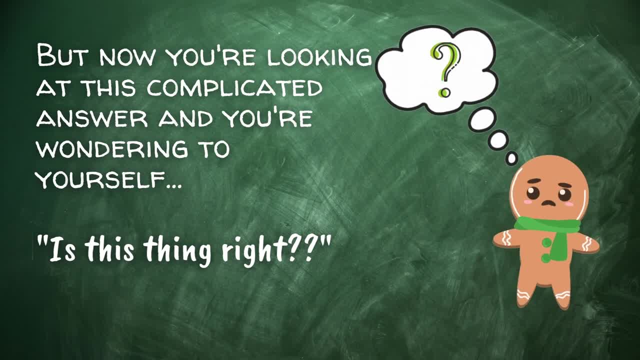 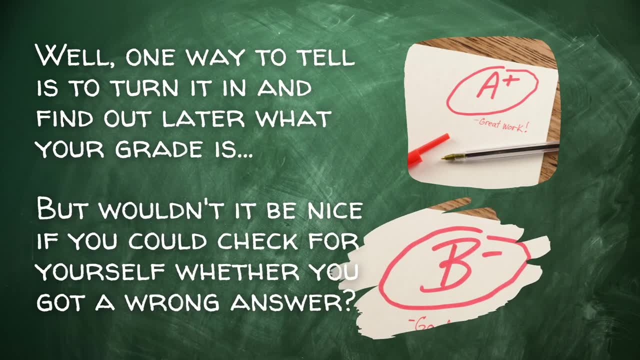 at this complicated answer that you've written down and you start to wonder to yourself: hang on, is this thing right? Well, one way to tell is to turn it in and find out later what your grade is. But wouldn't it be nice if you could check for yourself whether you got a wrong answer? 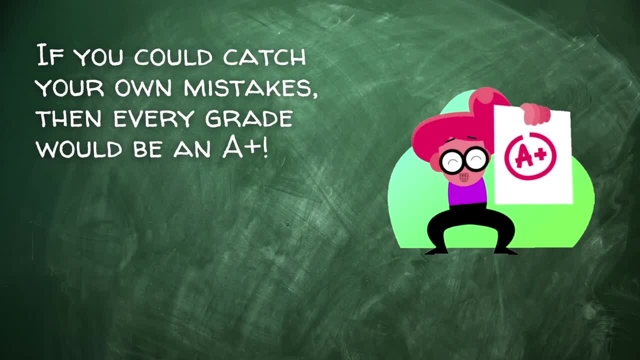 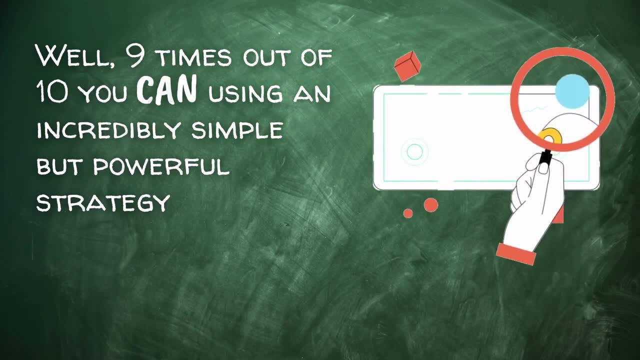 If you could catch your own mistakes before you turn in your work, then every grade would be an A+. Well, nine times out of ten you can catch your own mistakes using an incredibly simple but powerful strategy that beginning students don't always appreciate. I certainly wish I'd. 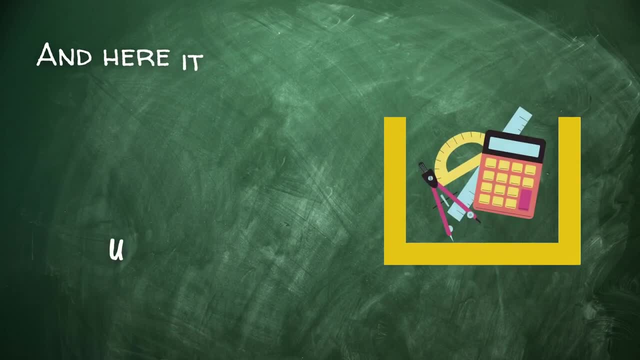 made better use of this strategy when I was a beginner. And here it is. Whenever you write down an answer before you put a box around it, you check that it has the right answer. And here it is. Whenever you write down an answer before you put a box around it. 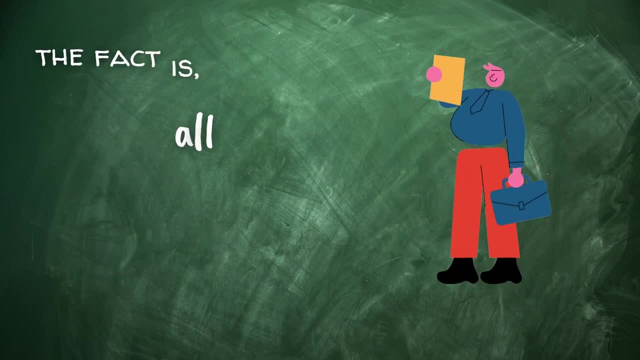 you check that it has the right answer. And here it is. Whenever you write down an answer before you put a box around it, you check that it has the right answer. So if you check the units of your answer and find that they're wrong, then you immediately know you must have made a mistake. 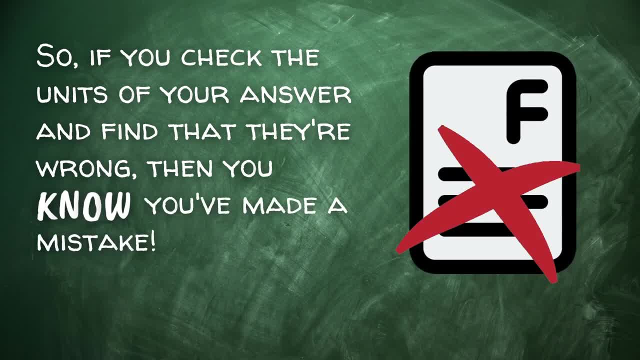 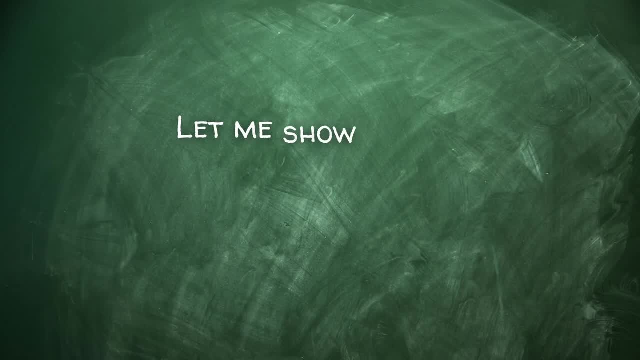 somewhere and you need to backtrack. That way, you can track down your own mistakes and elevate your grade. Let me show you an example of how this works. Let's take a look at this, niemand, and you don't need a regular week valve. The reason why this works is because, if we try to 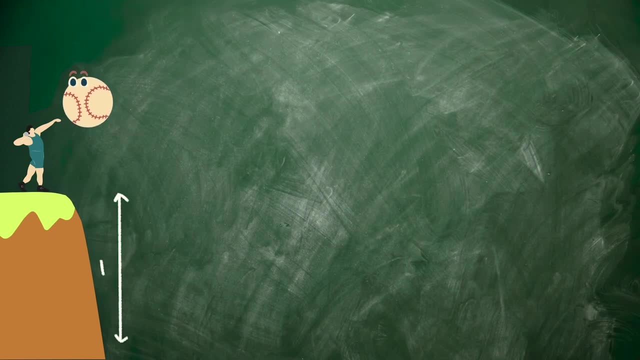 projectile motion problem. So we've got somebody standing on a cliff of height h and they throw a baseball at speed v and at an angle theta above the horizontal. So the ball is going to travel along this arc and the question we want to answer is: how far from the bottom of the cliff will the ball hit? 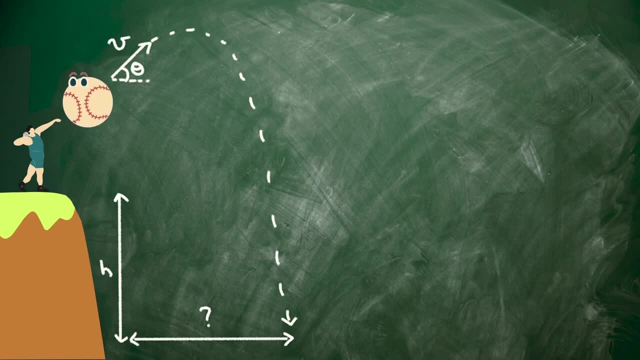 the ground. So how are we going to figure this out? Well, one strategy is to write down the trajectory x of t and y of t. Then, if we figure out where y is equal to 0, or- I put my origin at the base of the cliff here- if we evaluate x at the 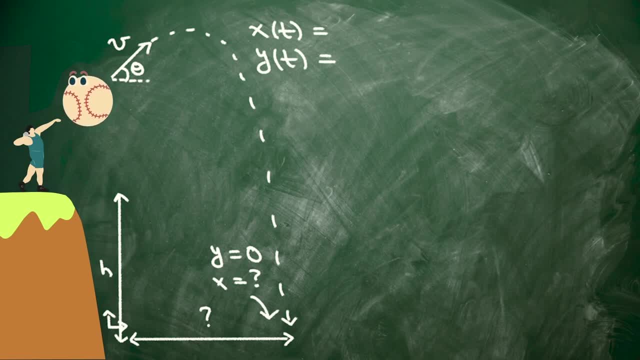 moment that y equals 0, we'll figure out where the ball hits the ground. So what is the trajectory? Well, remember that there's no acceleration in the horizontal direction, so the ball is just moving in the X direction with constant speed, whatever it had to begin with. That's v times cosine of theta, and so we. 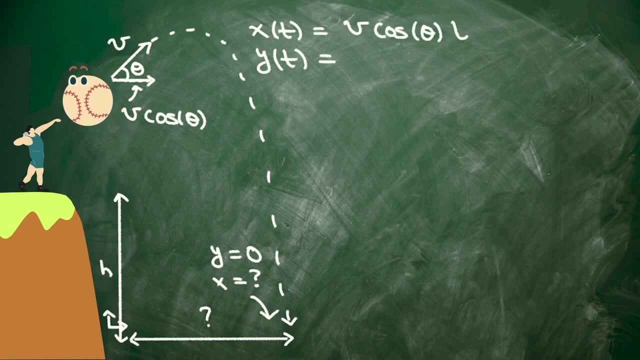 have: x. of t equals v cosine theta times t. Now, in the y direction, the ball has acceleration-minus g and it starts at height h above the ground. So the trajectory is h minus one half g t, squared plus the initial vertical velocity, that's v sine of theta times t. 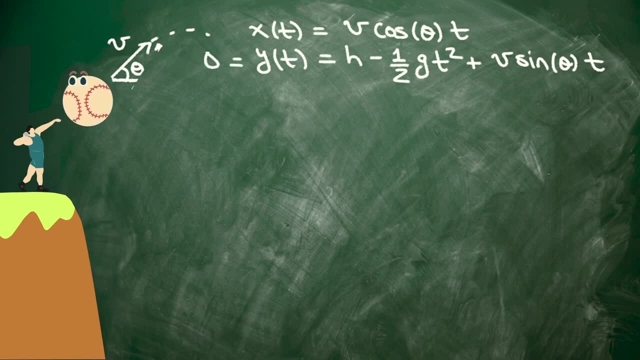 Now our strategy is to set the y coordinate equal to zero, solve for the time and then plug that in to the x coordinate. So we have a quadratic equation here for t, One half g. t squared minus v, sine of theta times t minus h equals zero, And we can solve using the quadratic formula. 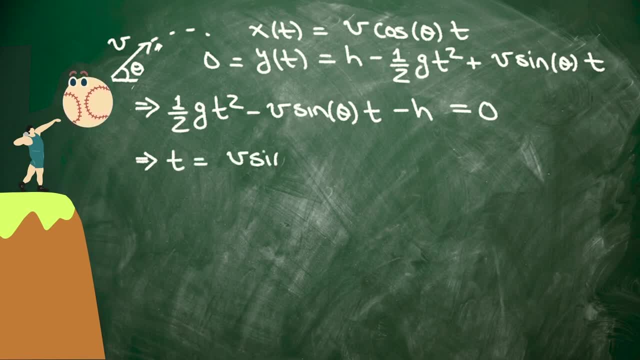 We've got: t equals negative b, that's v sine theta plus or minus the square root of b squared minus four a, c, that's v squared sine squared of theta plus two g, h. Now we want to pick the plus sign here because we want the time to be positive, not negative. So that's the time when the ball is. 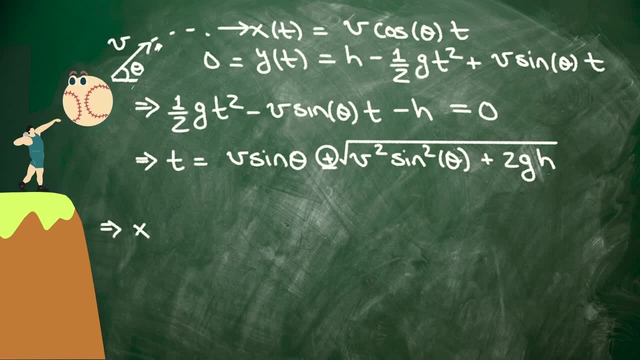 going to hit the ground. Let's plug it in to our x equation to figure out how far from the bottom of the cliff the ball will be. We've got v cosine theta times that time, v sine theta plus v squared sine squared theta plus 2, g, h square root. So that's our answer. but now, before we go ahead, 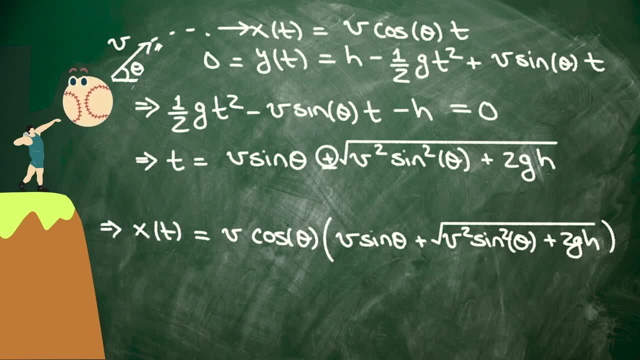 and draw a box around that and move on to the next problem. let's pause to check our units. We're looking for a distance here, x on the left, so our answer had better be in meters. Well, we've got v here, that's measured in meters per second, because it's the speed. 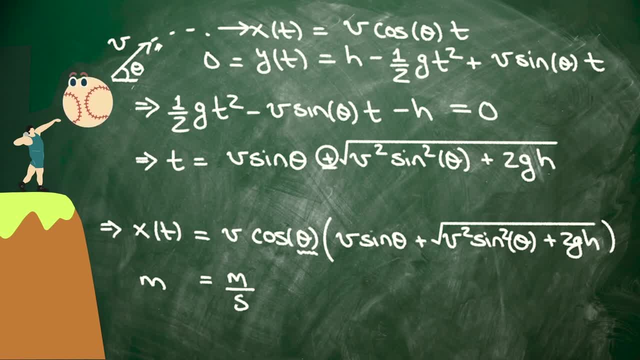 Theta is dimensionless, it doesn't have any units. Then inside the parentheses we've got v again, that's meters per second, plus this thing inside the square root We've got meters squared per second. squared from that v squared plus 2 g, h, The g is an acceleration that gives us meters. 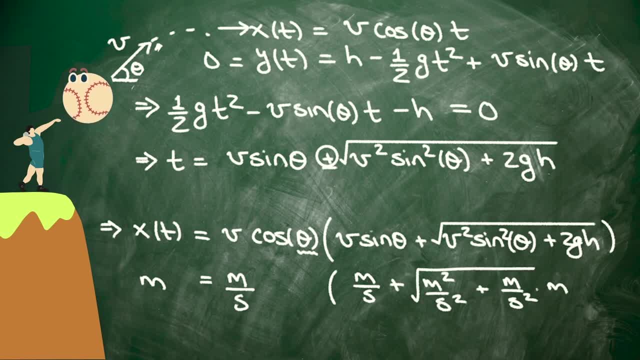 per second squared times h, that's in meters. So we've got meters per second inside the parentheses times meters per second out front gives us meters squared per second, squared all together on the right hand side. Now the alarm bells go off. The fact that these units don't match up immediately tells. 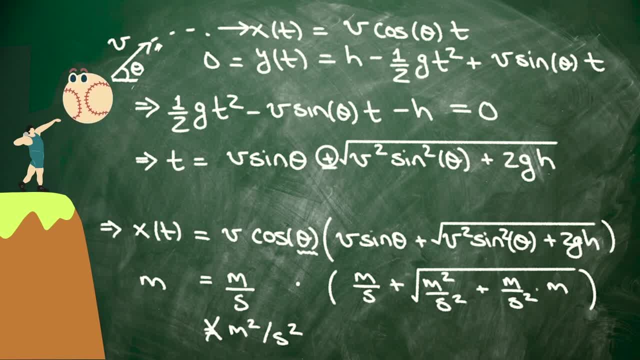 us that we must have made a mistake. So now we want to backpedal a bit to try to find out where we went wrong. This quantity- in parentheses- that has units of meters per second- that was supposed to be the time that it takes for the ball to hit the ground. So evidently we must have 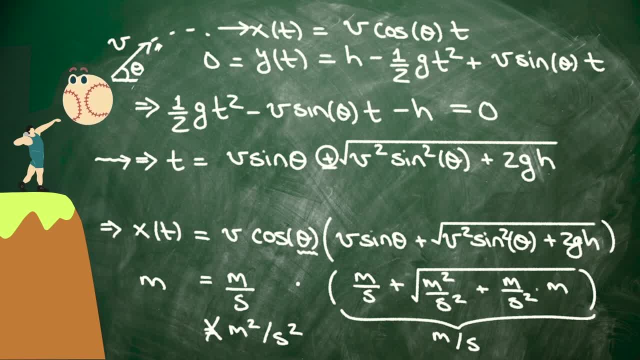 something up when we wrote down our formula for t. We were supposed to get seconds, but instead we got meters per second. t was the solution to this quadratic equation. We had t equals negative, b plus or minus, the square root of b squared minus 4ac over 2a. That was the mistake I forgot to. 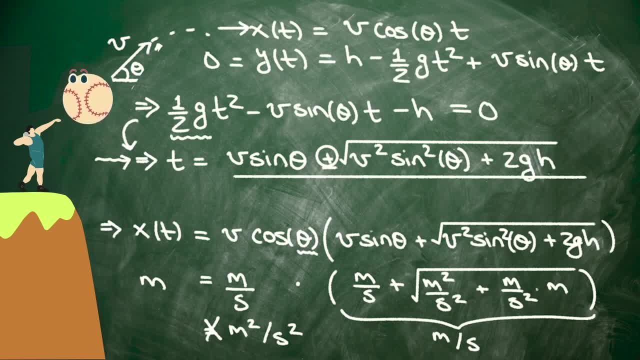 divide by 2 times a, which in this case contributes a 1 over g, So that 1 over g changes the formula for the time to hit the ground and therefore it changes the horizontal distance covered. g, remember, has units of meters per second squared, So when I take 1 over that it flips. 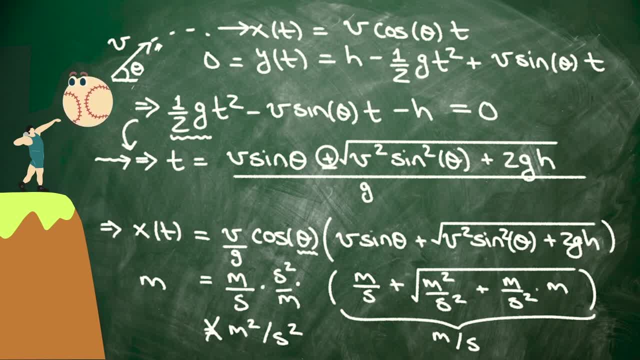 it over and I get seconds squared per meter. So all together, we've got meters per second times seconds squared per meter, times meters per second. The meters cancel, the seconds squared cancel and lo and behold, we're left with meters, which is what we wanted. We were able to catch our 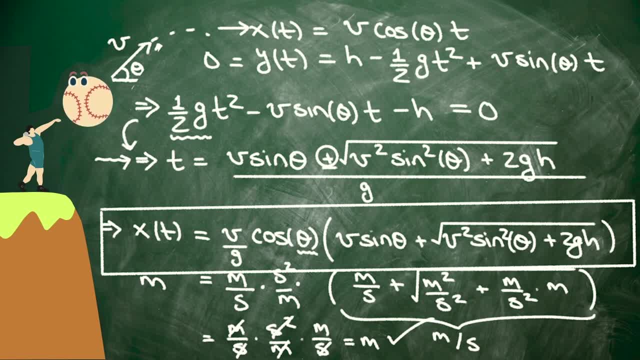 algebra mistake by checking the units of our final answer. Now, checking the units doesn't get us anywhere. We can't get the units of our final answer. We can't get the units of our final answer. For example, it doesn't tell us that we got these factors of cosine, theta and sine. 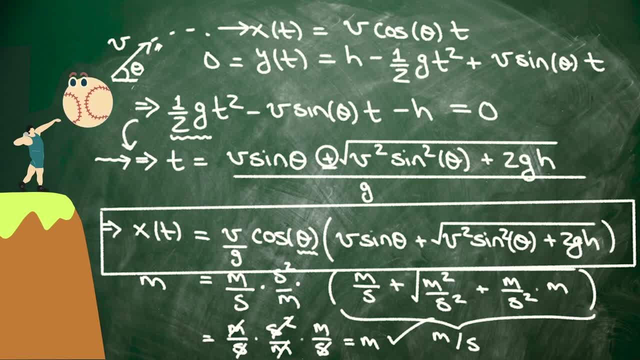 theta correct because those factors were unitless. And likewise there could be factors of 2 and half and pi and so on. that we can't get just by looking at the units. But whenever you have the wrong units you know for a fact that you had the wrong answer. There are additional checks that you can. 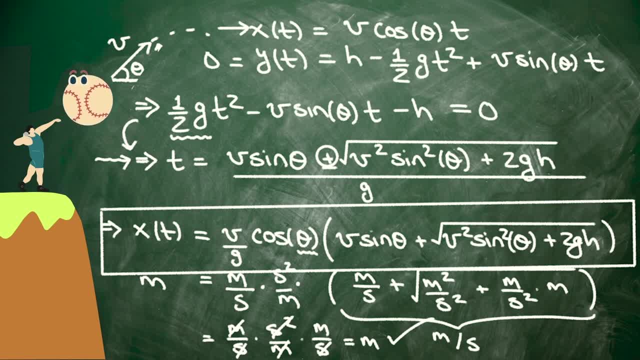 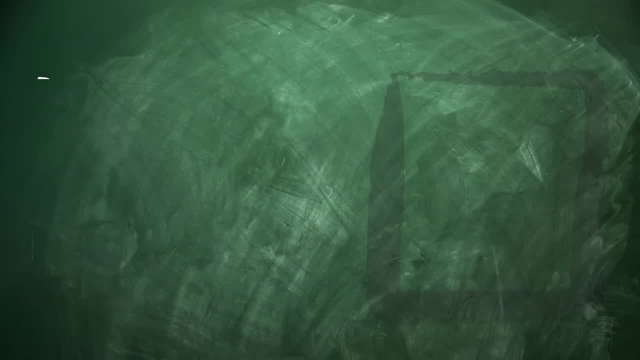 make to see if those unitless factors make sense, like checking a limiting case. I'll show you how that works in a future video, so make sure that you're subscribed to the channel. So the thing that I hope you'll take away from this video is that, by double-checking your units, 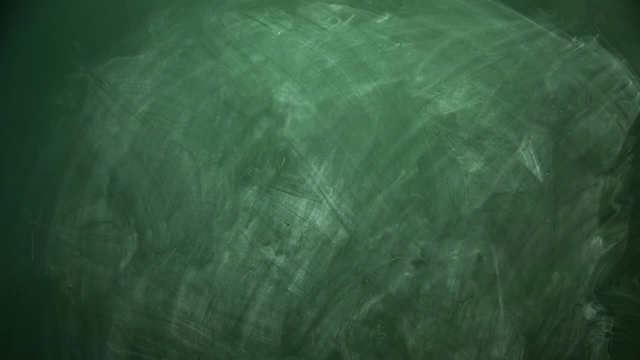 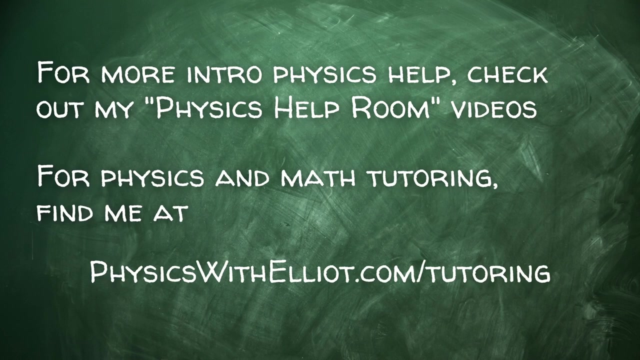 you'll be able to catch so many of your own mistakes, You'll get better at physics and your grades will go through the roof. So I hope you found all that useful. For more help with your intro physics classes. you should check out my physics help room videos here on the channel.